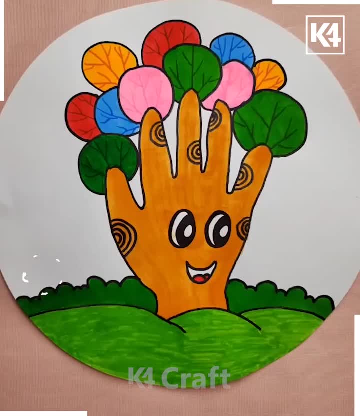 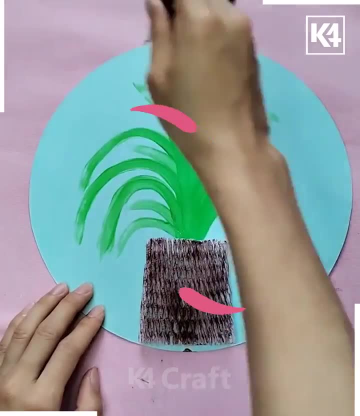 It is ready, Isn't it looking amazing? Yes, Damn, it is Proceeding in this way. let's see. what are we going to do now? You just have to take the pieces like this and then, with the help of watercolor, you have to paste it in this manner. Now, what you have to do? you have to give the 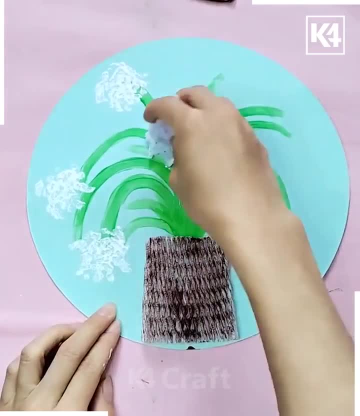 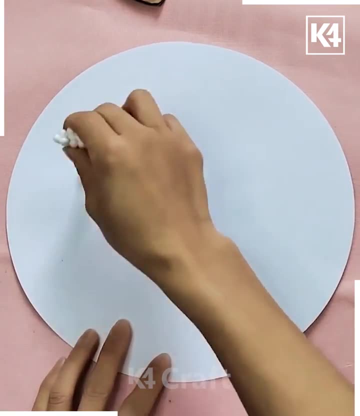 imprints like this using the paper, and then you will get an amazing, beautiful picture and, again with the help of earbuds, you can put the yellow dots in the middle. Proceeding in this way, you have to give the impressions with the help of watercolor like this, with the help of: 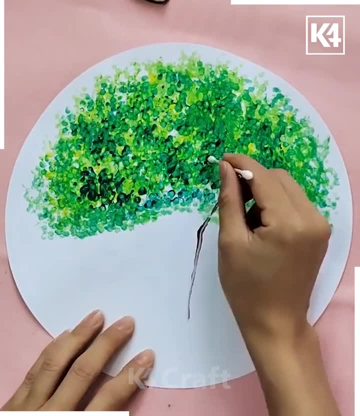 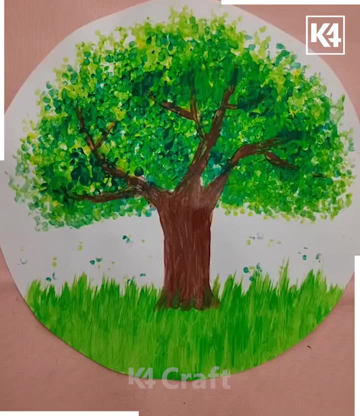 group of earbuds and then you will get an beautiful result. keep on making this and then the branches of the tree handling from the top. you just have to make it like this again. you can give it a final touch. keep on proceeding in this way and let's see what are we gonna make. just make the imprint circular spiral. 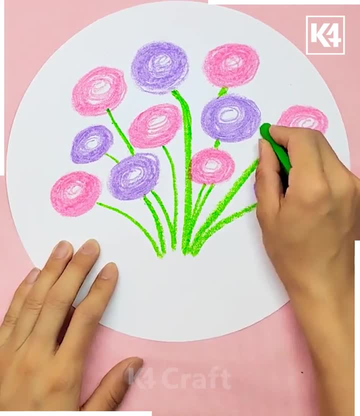 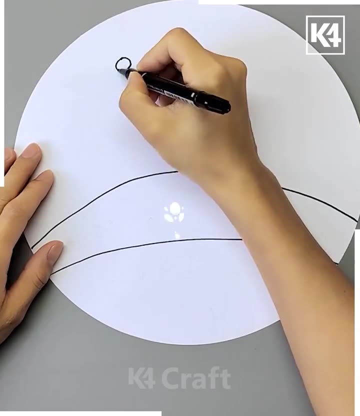 imprints like this and join it like this with the help of oil, pastel colors. make the leaves around in this manner and make a basket and paste love on it. proceeding in this way, you have to make the curvy lines like this, and again you have to make the petals of flowers in this manner. join it further and you will. 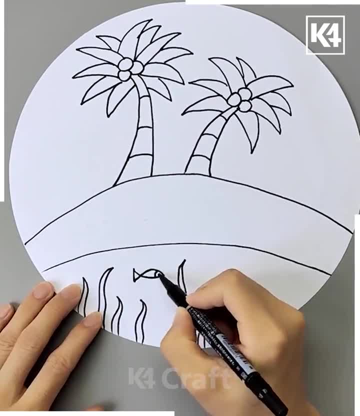 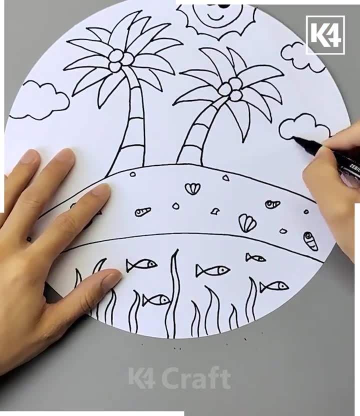 get coconut trees like this. you have to make the view of a beach you have. you can decorate it further by coloring it and proceeding further in this manner. keep on making the patterns and your drawing is absolutely ready. now, with the help of clay, press the place like this all over the body and let's see what are. 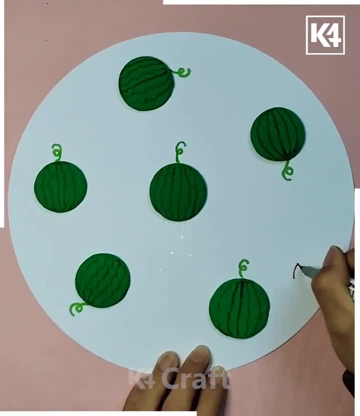 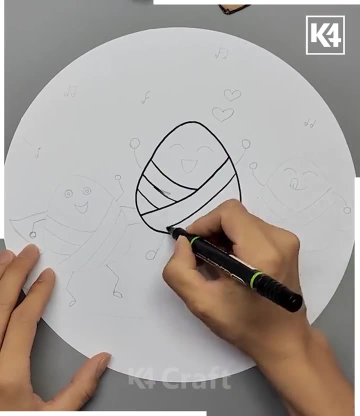 we going to do you. with the help of black marker, you can make imprints like this and your watermelons are ready. you can give it final touch. proceeding in this way, you have to make the petals of flowers in this manner, join it further and make the cartoon character in this manner, make it look like this and again. 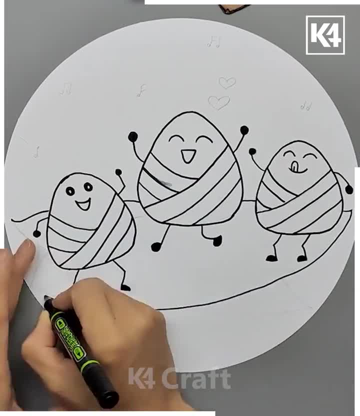 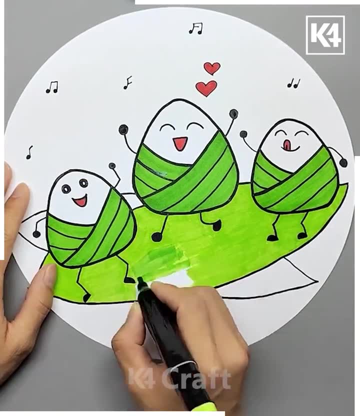 you have to make this doll dancing doll in this manner and then decorate further by making it look colorful and interesting. you can just give it a beautiful look like this and your scenery is damp, ready to go. you can just make it look for their amazing proceeding in this manner. make a pot. 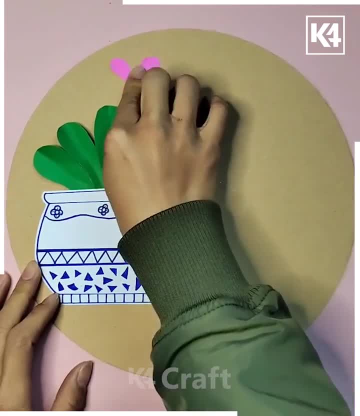 like structure and then paste the leaves inside it, and then, with the help of play, you have to give the imprints in this manner and you will get a beautiful, amazing result. will to help how you can give it a final touch, and here I just need a spider web.